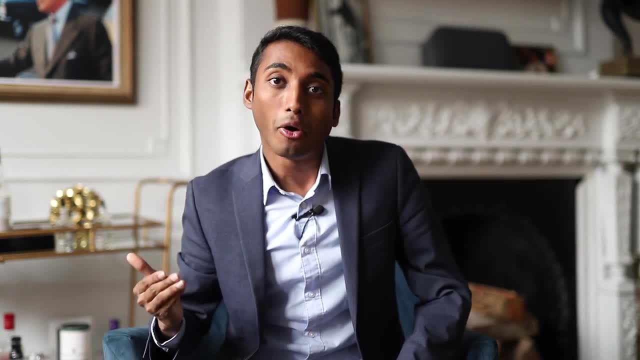 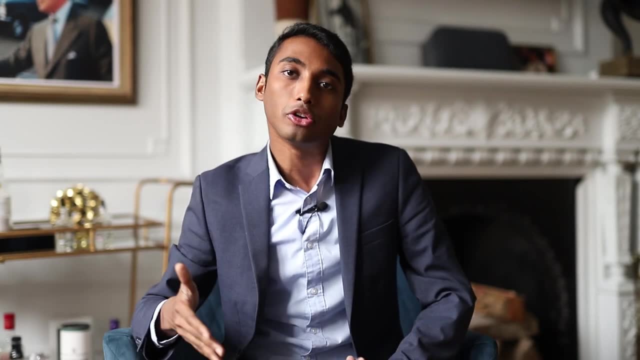 the marathon And if your friend knocks on your door at 5 am, boy, are you going to get out of your house and run that marathon. But with public speaking it's a lot more trickier because it's harder for you to do those types of exercises without that clear. 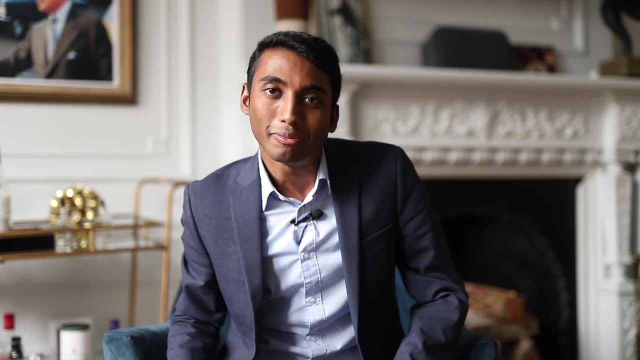 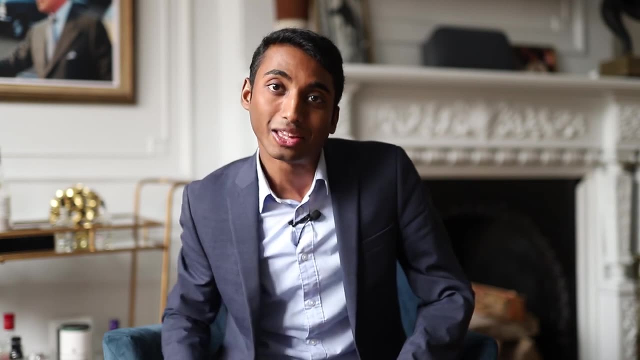 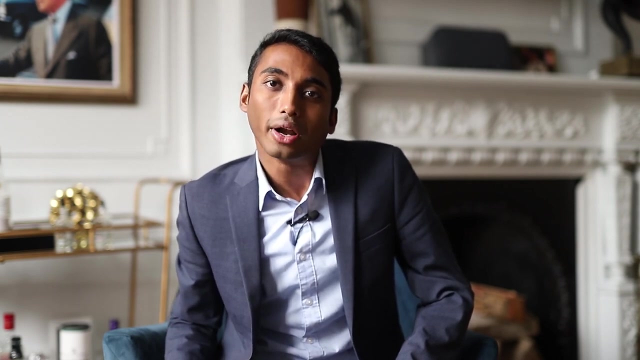 goal, And that's exactly why, in this week's episode of MasterTalk, we'll be elaborating on my three daily exercises to help you master your talk on a daily basis. Hi everyone, I hope you're having a fantastic week. Brendan from MasterTalk, here and today we're talking. 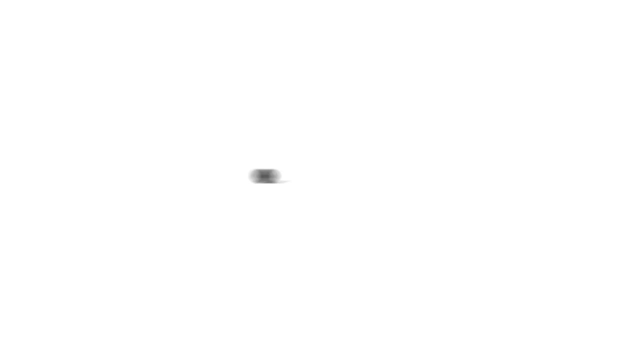 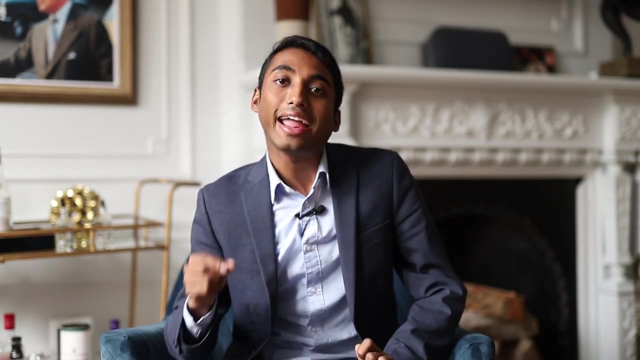 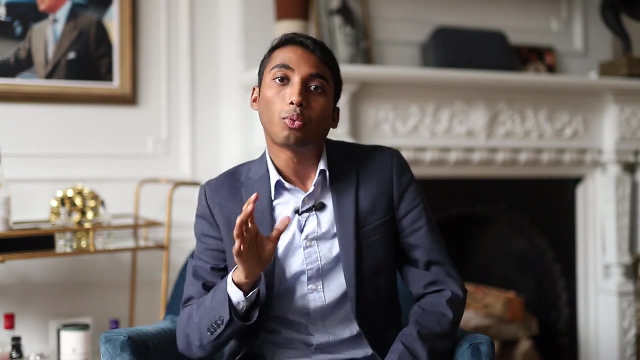 about the daily practices, So let's get into them. Number one: the random word exercise. I absolutely love this word. I love this drill because if you can master it, you'll be in the top 1% of public speakers. The random exercise is simple. All you do is you have a friend, give you a random word. 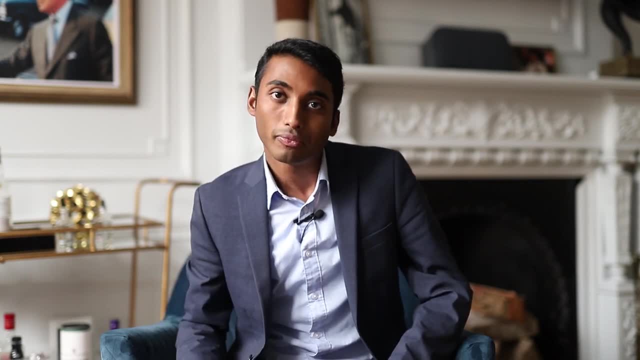 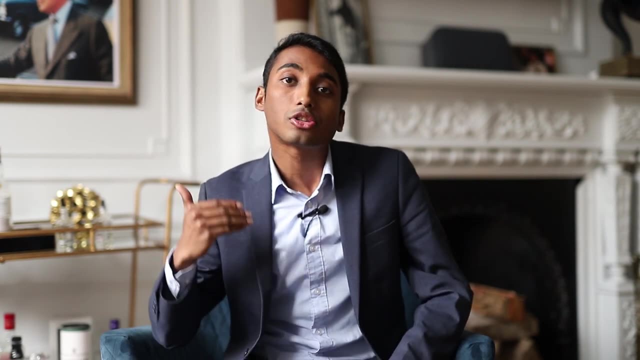 in the dictionary that you need to then build an introduction from. This is very interesting because if you're able to master this, you'll have a lot less stress in presentations. You'll also learn to think on your feet more faster and you'll be able to give presentation like 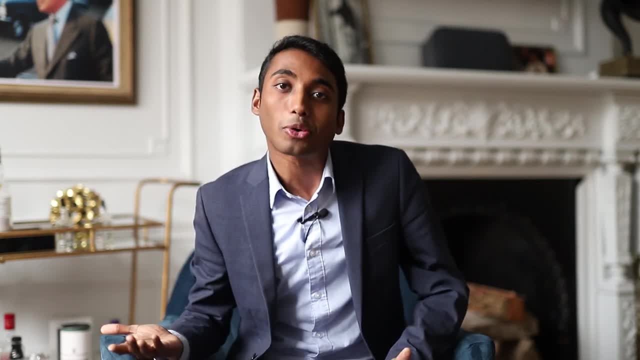 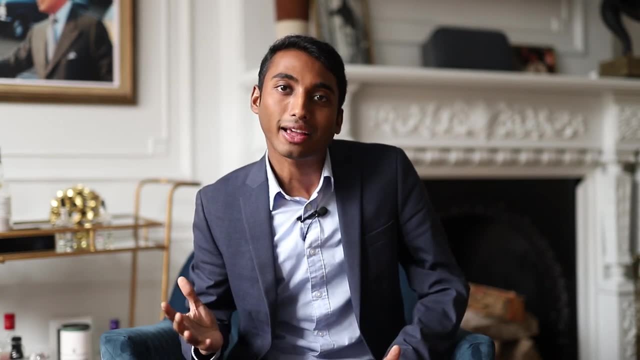 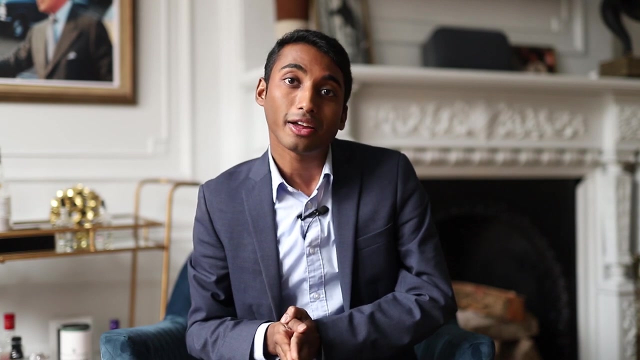 spontaneous ones, specifically out of the cusp. I know this is a recording and I might be cheating, but let's use camera as an example to demonstrate this. Shots, The shots that you take, aren't just pictures. They're experiences, They're moments that don't just last for yesterday. 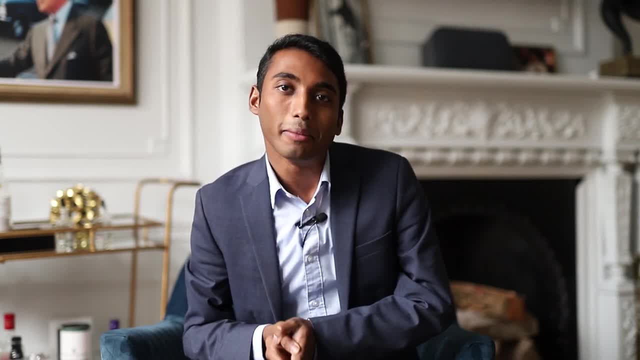 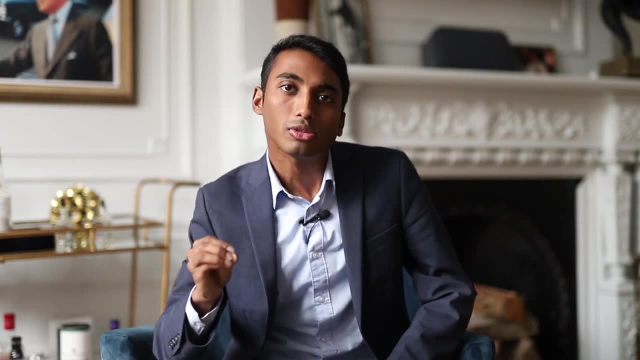 for today or even tomorrow, but for a lifetime of shots, As you can see from the way that I just created a random introduction from camera. you can then use that for multiple different words and practice five words for five minutes every single day, And that's. 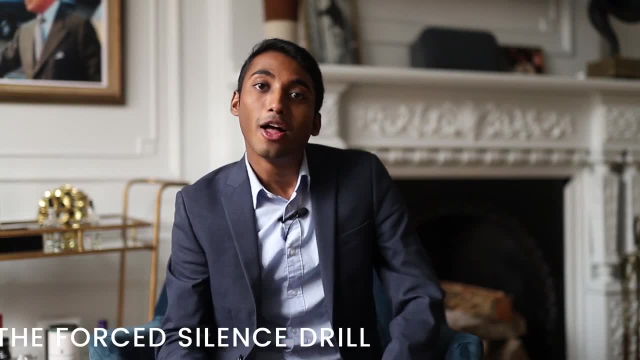 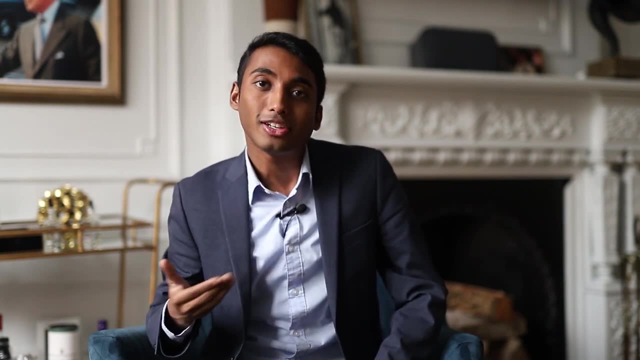 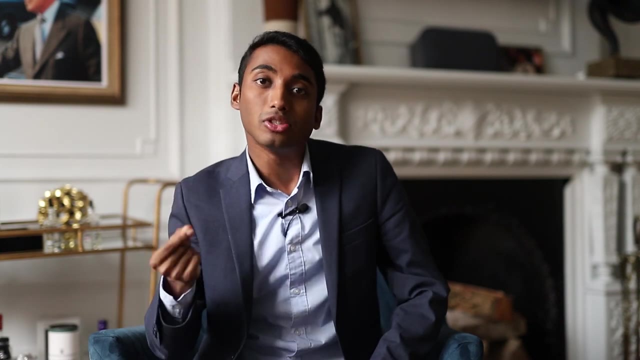 what we're going to do today, So let's get started. Number two: forced silence drills. The biggest difference between great speakers and exceptional ones is their ability to use silences as a way to make their presentations better, and forced silence drills help you make those differences by making your silences better. 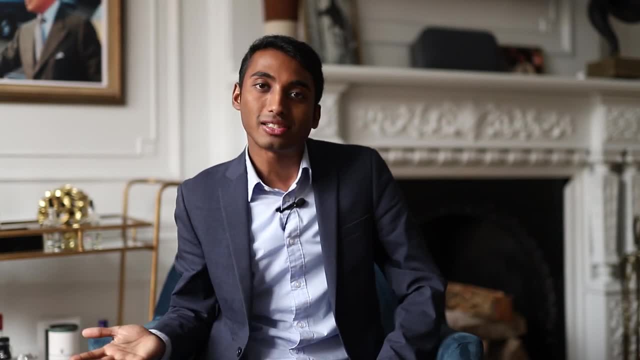 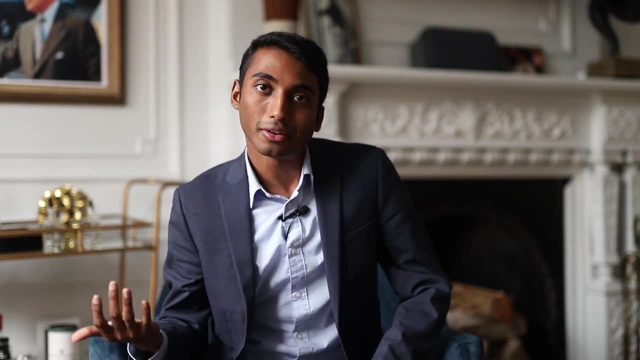 and more strategic in your presentations. So the exercise is very simple and it's a lot easier to do with a partner. All you do, as you have a partner record, you give a presentation right. So you're giving a presentation for a minute or two and then, in the second recording of